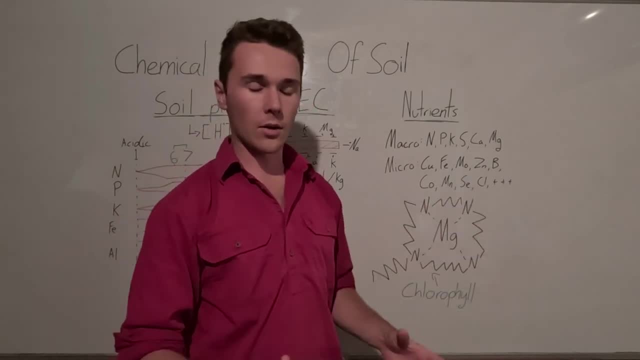 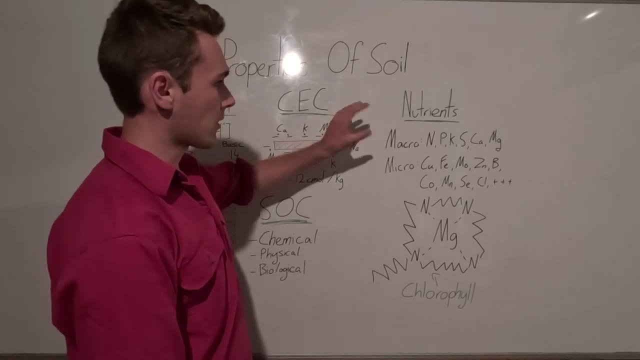 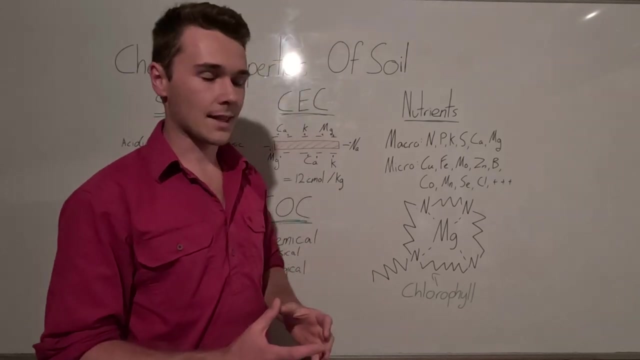 take up these nutrients to build the body of the plant, And so we can break down our nutrients into two different categories. We have macronutrients and micronutrients. As the name suggests, macro means large, So we need these nutrients in large supply, And micro is the nutrients we need. 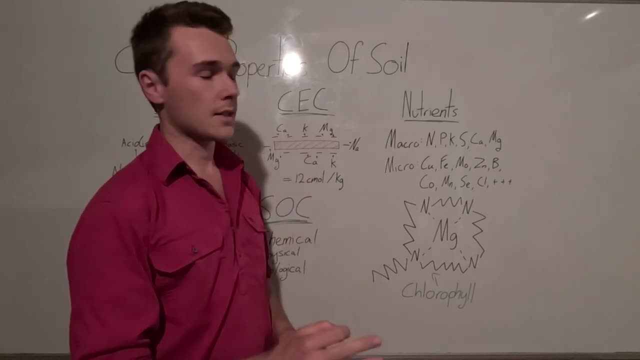 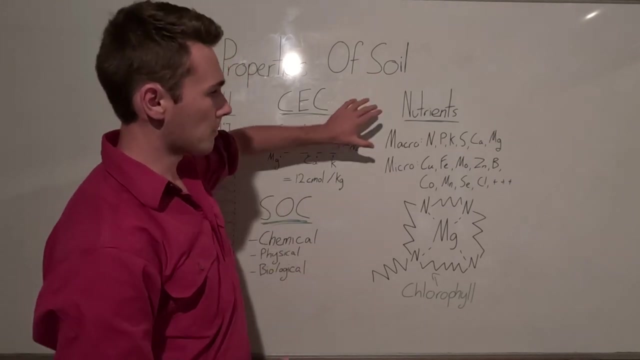 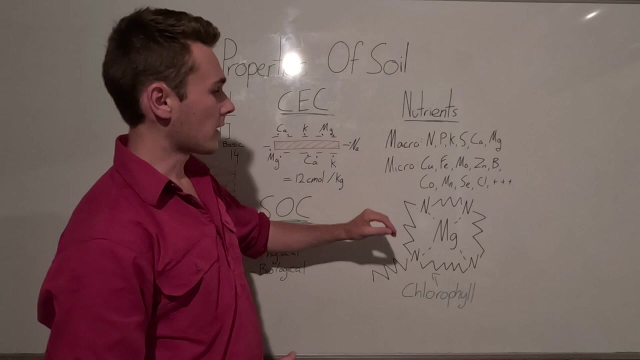 not in large supplies, just in sufficient amounts so that we can function as usual. It's interesting when you think many people think you know macros are they're more important than the microbes and the micros, but they're actually just as important as each other, And if you're missing just one of these, 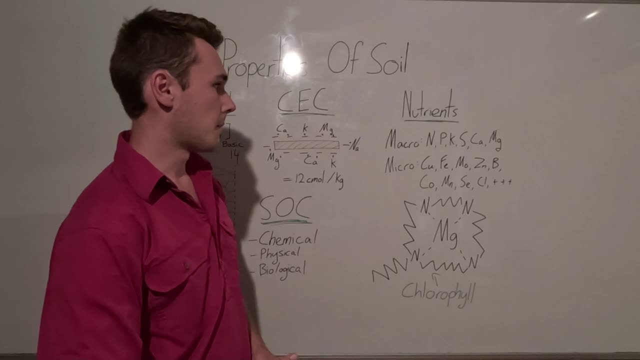 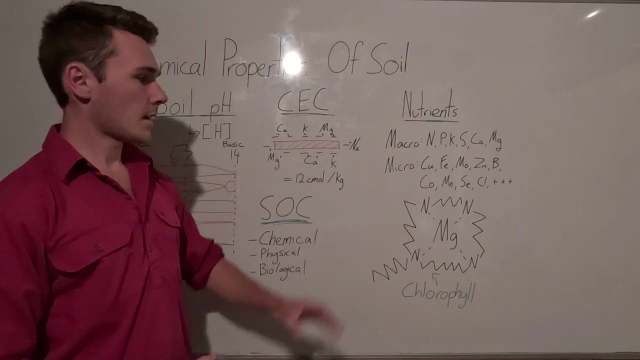 micronutrients, your plant doesn't function as well and it's going to be limited by that nutrient. So they're all important, just the amounts change and it depends on the nutrient, And so each of these nutrients will have a particular function in our plants. Now also, it's important. 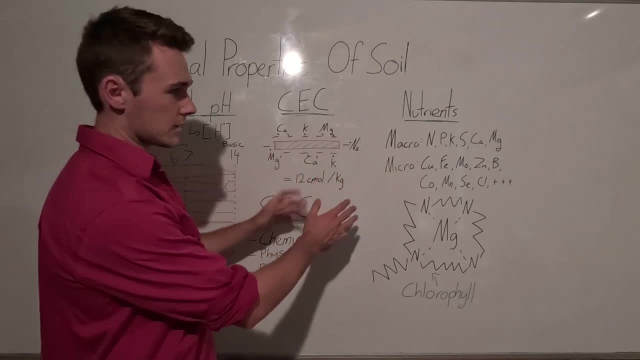 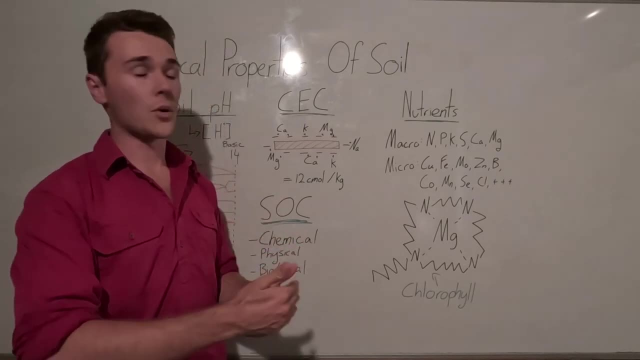 to mention. it's a lot more plant nutrients than I've just listed here, And it's coming out every day that more and more nutrients are essential for plant development. but it might just be in a very small amount Now when we refer to essential nutrients. 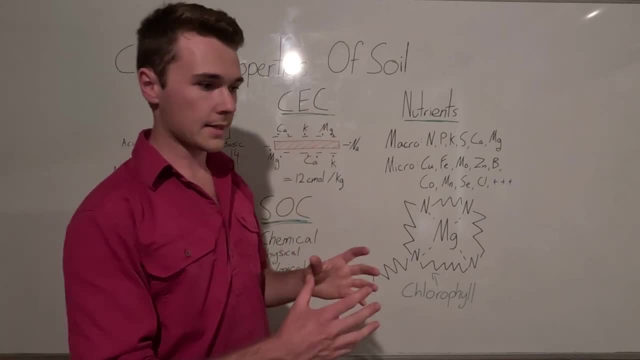 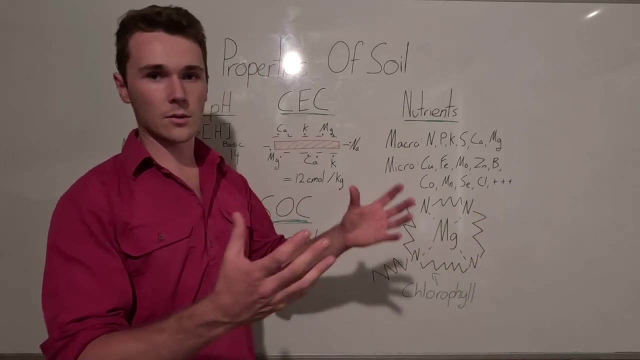 it means that the plants, firstly, can't replace the function that the nutrient plays in the plant. So if a particular nutrient plays the role of building cell walls, like calcium, no other nutrient can replace that nutrient, And so it's essential that the plant has that. 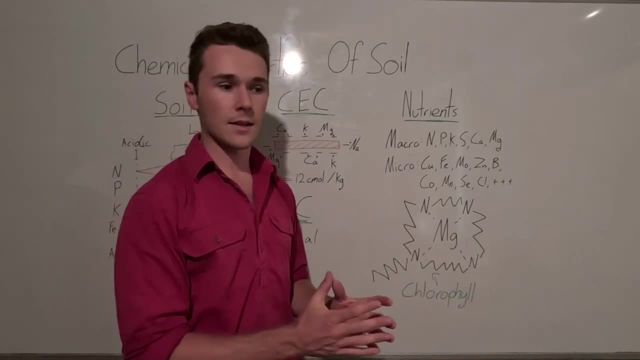 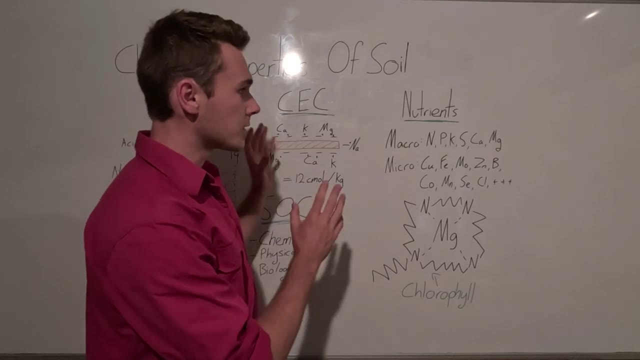 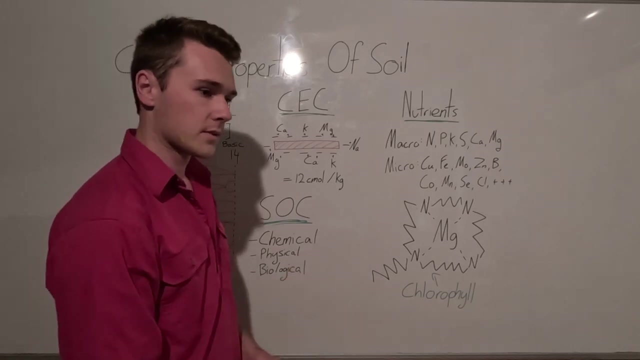 nutrient in order for it to fulfill that function. So if there's none of that nutrient, it then can't do the particular function. There's no substitute. All of our soil chemistry really evolves around these nutrients, how they interact, how they interact with our plants, how the soil, the physical parts of our soil, interact with these. 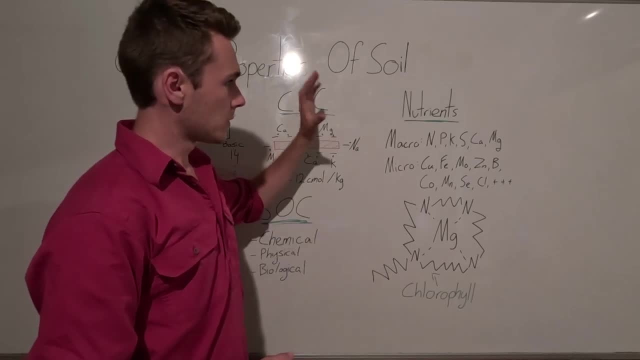 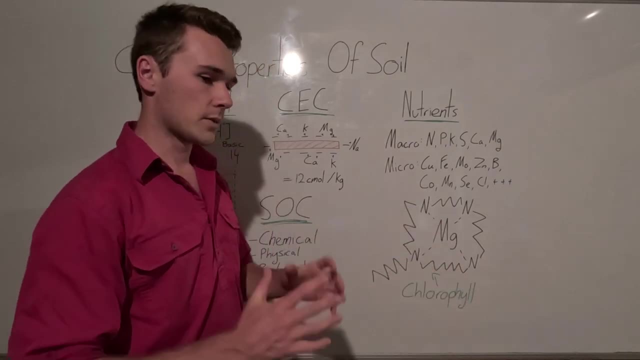 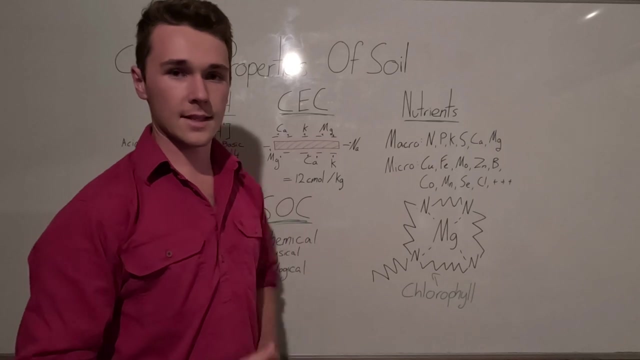 nutrients. Now, to some extent, the nutritional profile of our soil is largely given by the mineral makeup of our soil. So we have soils that are quite high in fertility, like our clayey soils, and then you have soils low in fertility, such as our sandy soils. So 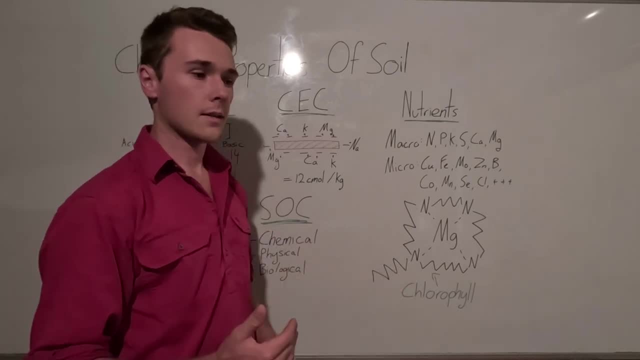 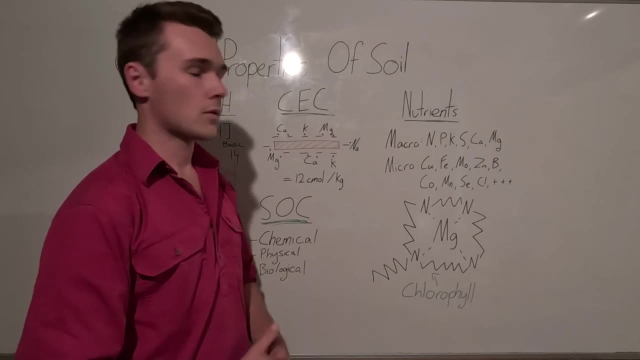 typically we have a lot of our fertility, given by the mineral component of our soil, And if we're lacking in any of these, we need to then supply it or rely on our soil. So if we're lacking in any of these, we need to then supply it or rely on our microbes to supply the plant. 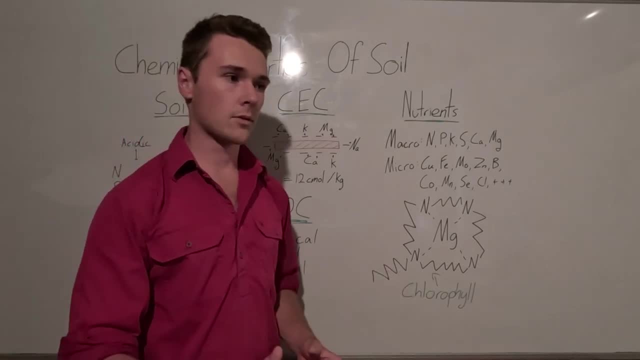 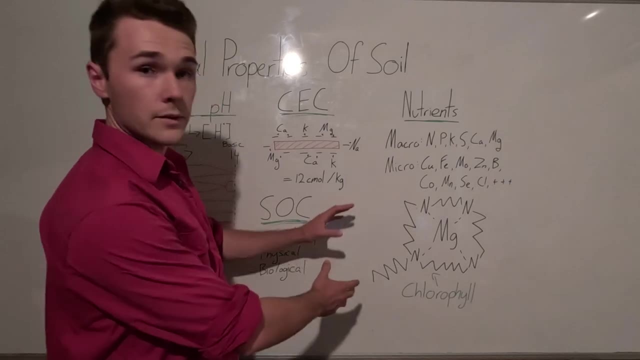 nutrition. So one way we can think about the importance of plant nutrients: think of it as like you're building something with Lego. So say, for example, we've got chlorophyll here. Chlorophyll is important for capturing light in our plants. This is very important for 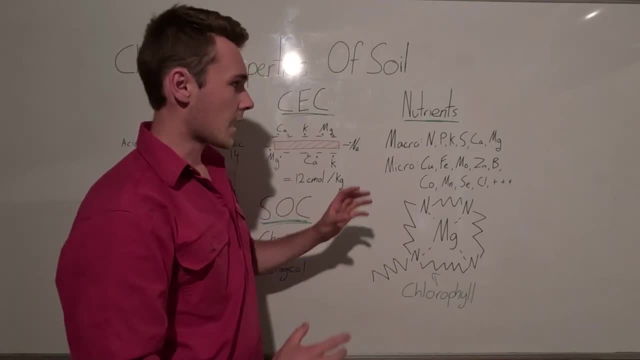 photosynthesis. You can see these swiggly lines here. They're just a carbon backbone for this molecule. You'll notice that we have four- nitrogen and magnesium- And so if we were to try and build this, but we didn't have magnesium, 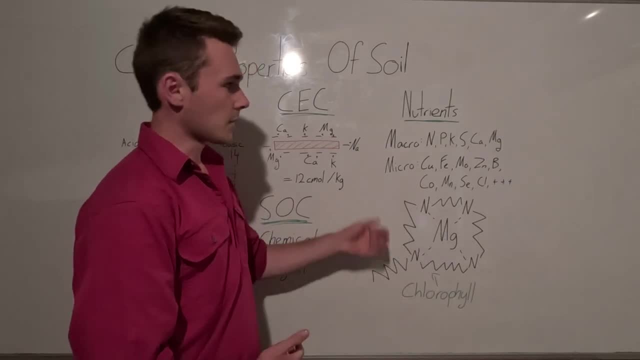 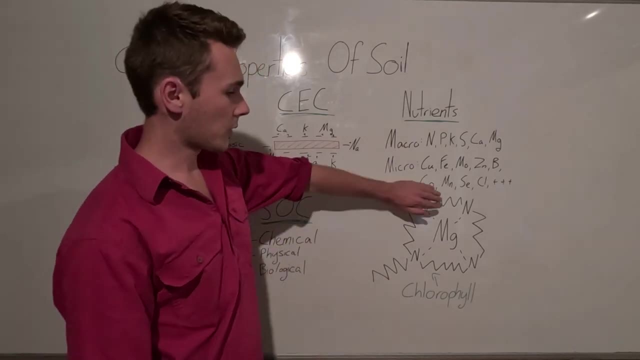 the compound just wouldn't work, And so, as I was saying before, we need a lot more macros than micros, but they're still just as important as each other. So if we only had three nitrogen, it wouldn't work. If we had no magnesium, then it wouldn't. 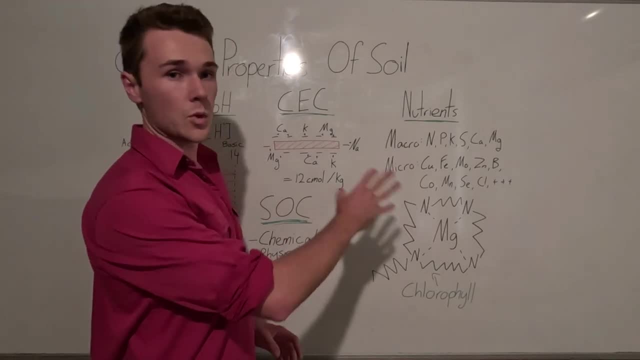 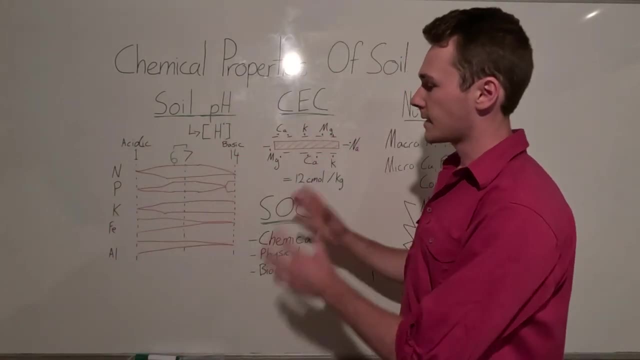 work, And so they're all important and they're all going to be available to our plant so that they can build their bodies. So let's go to our soil pH Now. soil pH: one of the massive things about soil pH is that it determines the availability of a lot of our 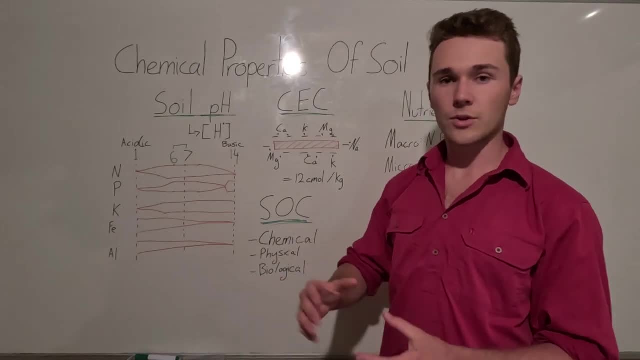 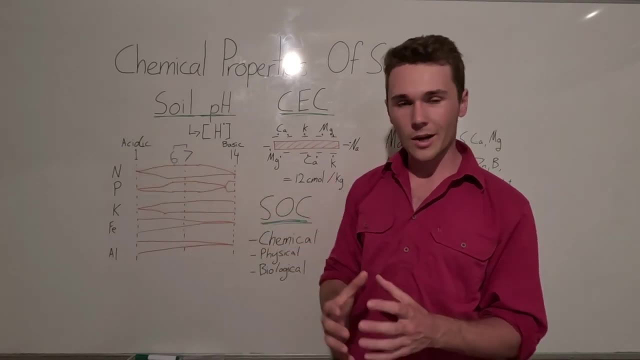 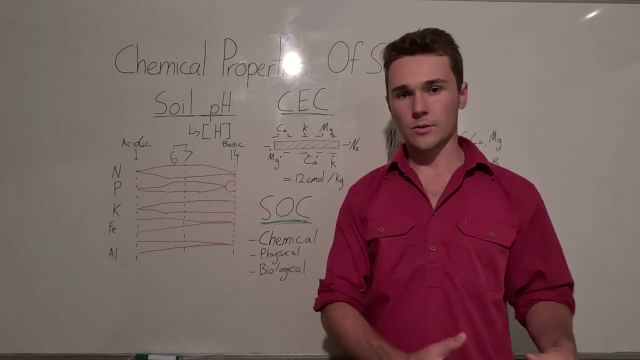 soil nutrients. pH in itself is the concentration of hydrogen ions and it is expressed on the pH scale, going from one which is highly acidic, which is a high concentration of hydrogen ions, to a basic soil which is very low in concentration of hydrogen ions, And that's expressed as a 14 on. 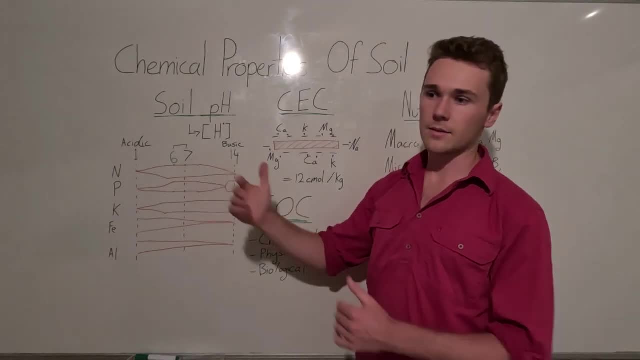 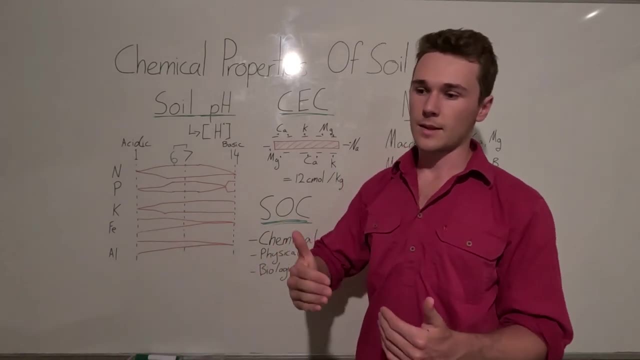 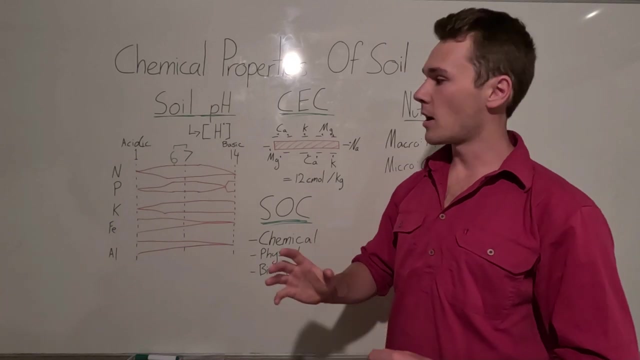 the pH scale, Logarithmic scale, which means the higher or the more hydrogen there is, the lower the score, and it's also logarithmic. So there's a factor of 10 difference between each of these. Now, each nutrient or element will have a different behavior at different ends of this spectrum. So 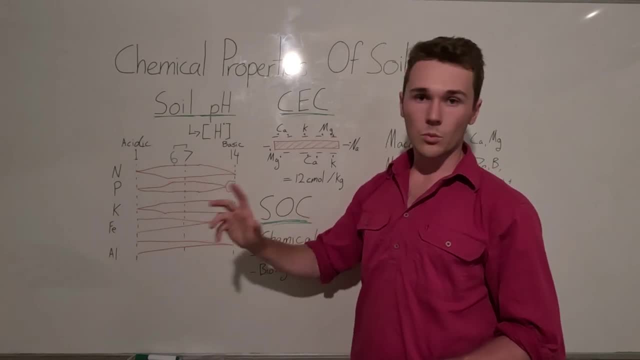 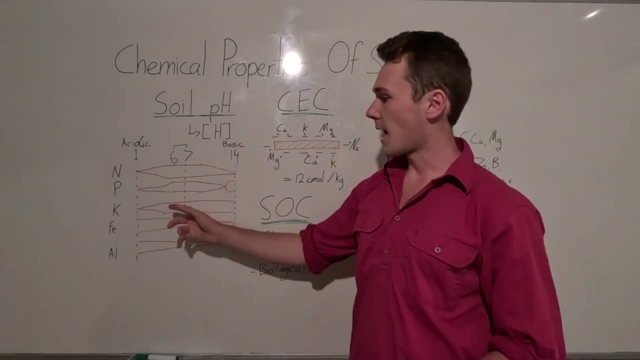 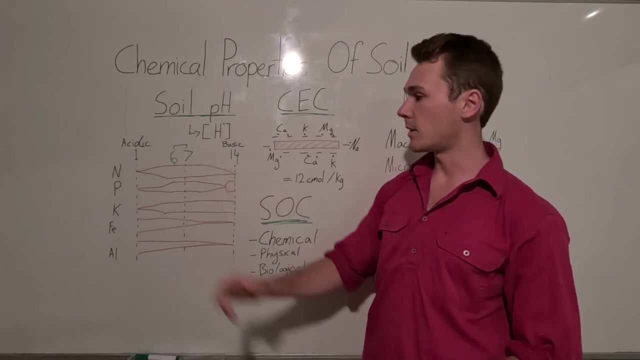 nitrogen, for example. it's pretty abundant around the seven, which is neutral, But once you go to either end of the spectrum the availability starts to decrease. It's interesting because phosphorus is similar, but it spikes here at the end. So the thickness of these lines represent the availability. 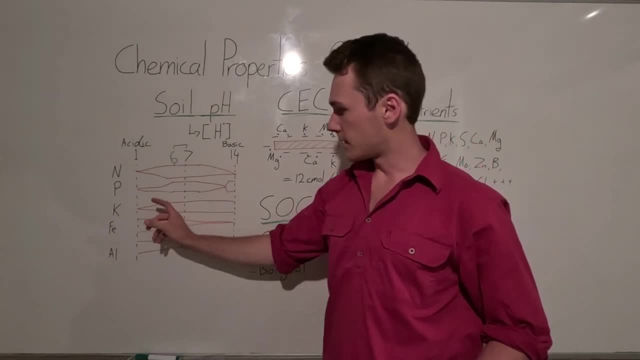 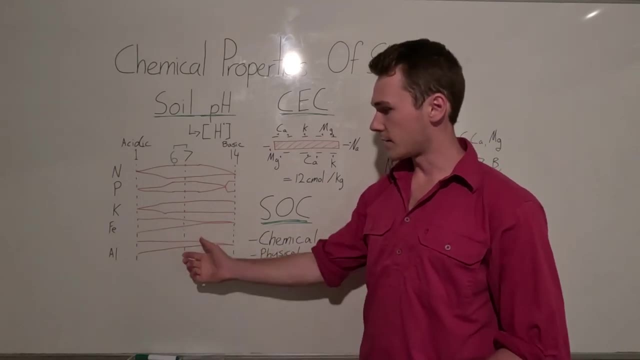 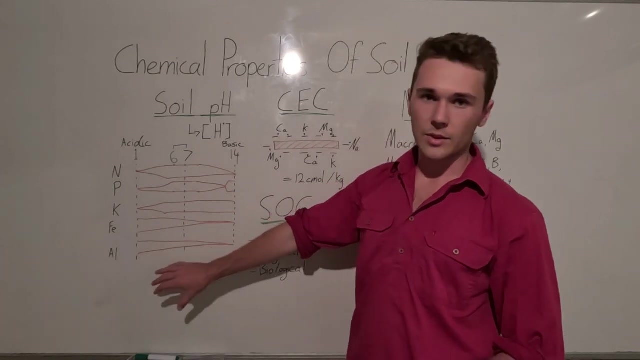 of that nutrient, Potassium, is pretty low availability when the soil is acidic, but increases as it increases in pH, and iron is the same. Now all this works with our nutrients, but it also works with anti-nutrients, such as aluminium. Now aluminium can become toxic to. 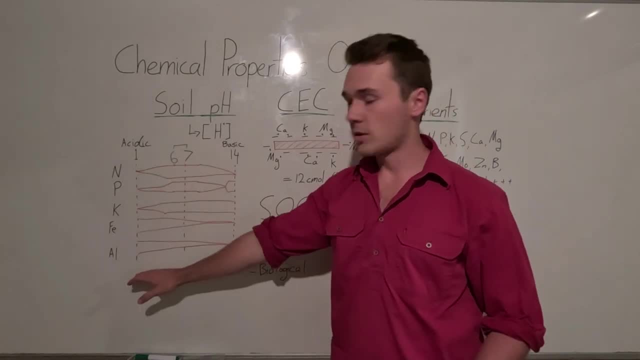 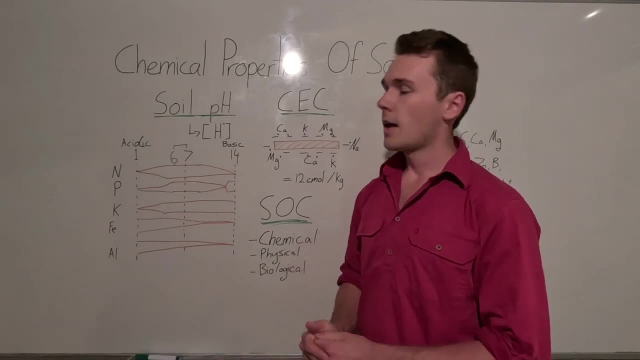 our plants, and so when we have a really low pH, aluminium increases the amount of sodium that's in our plants. Aluminium increases in its availability and can poison our plants. So sometimes our plants might seem to be deficient in a particular thing. Although that's correct and the plant actually might be deficient, it doesn't mean the soil is. 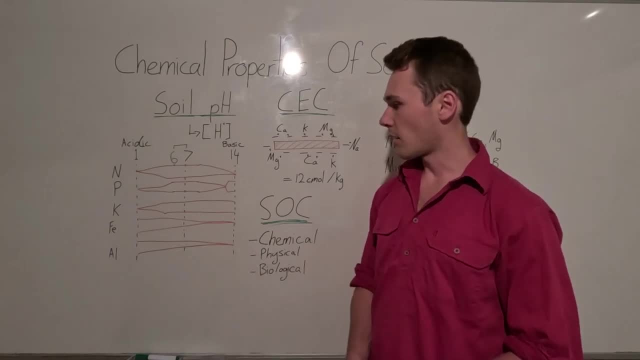 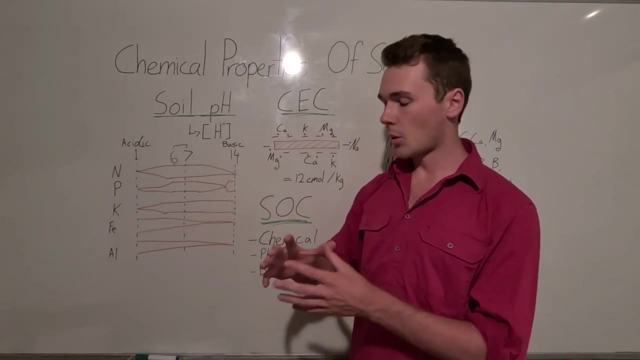 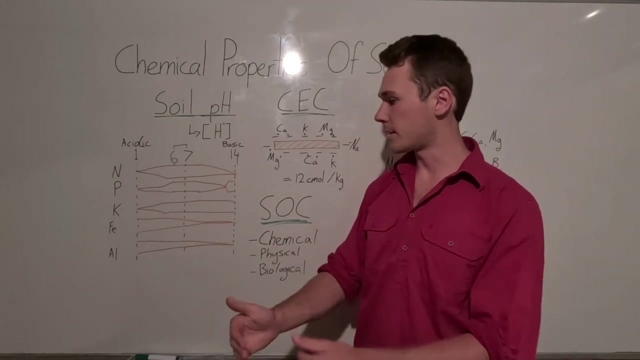 deficient itself with that plant nutrient. And so, for example, if we take iron, for example, if our plants are iron deficient, the soil doesn't necessarily need to be iron deficient. it might just have a high pH, which means the iron itself is not available to our plants. 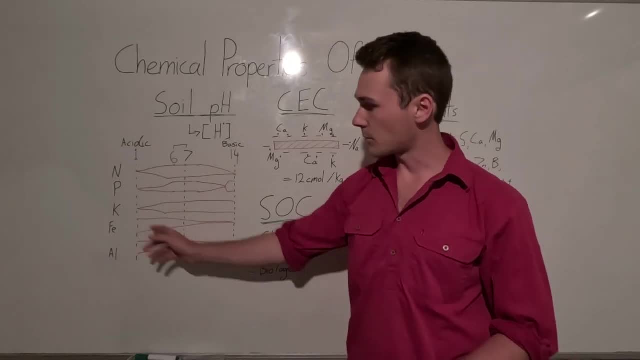 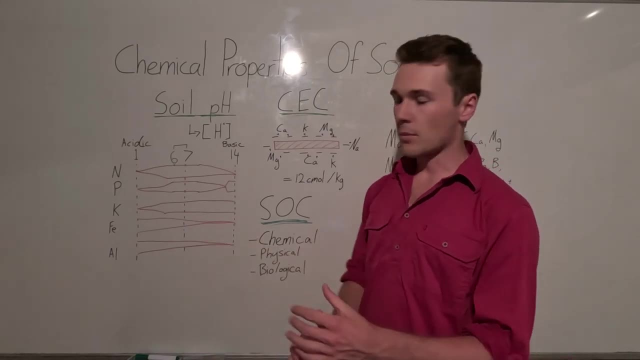 And so a management strategy that we can do is by lowering the pH we can increase the availability of iron. Now, the actual chemistry as to why different elements become more and less available at different pH is pretty complex, And I don't fully understand it. 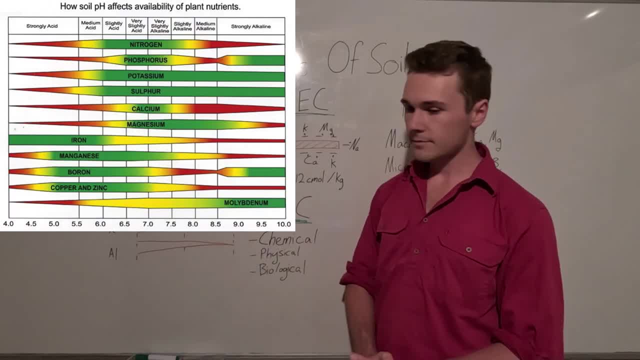 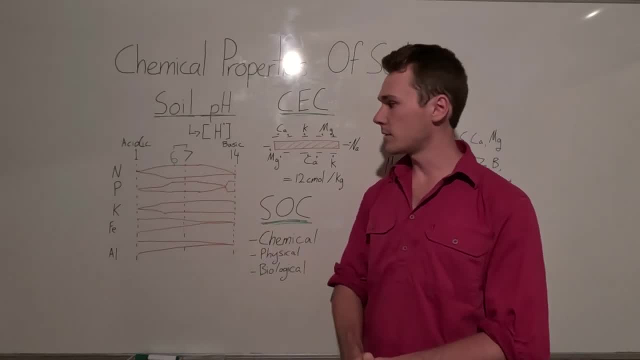 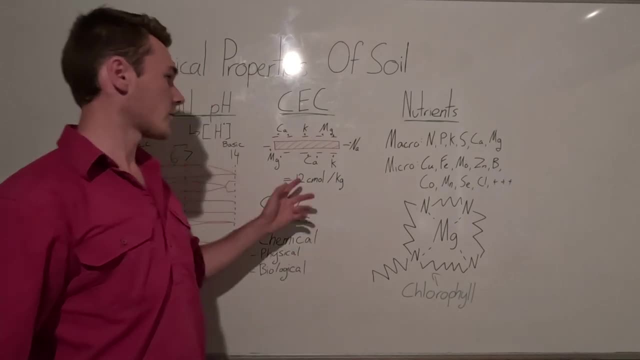 But as a general rule, here are the availabilities. with pH Again, we want to keep our soils between 6 and 7. That's ideal, And that is also where microbes can function the best. Another chemical property of our soil is our cation exchange capacity. 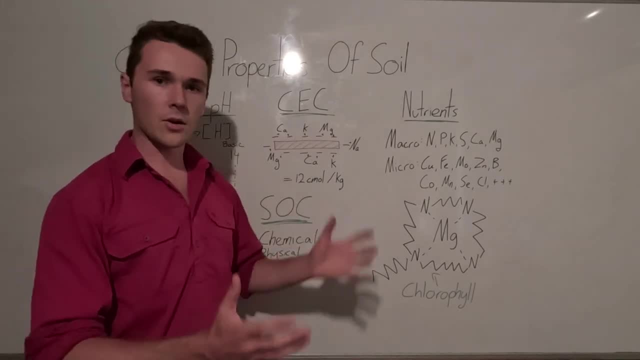 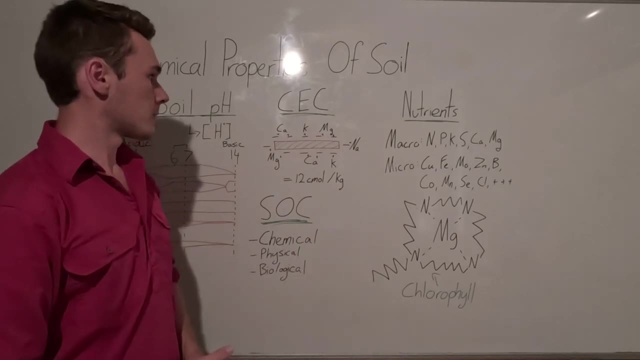 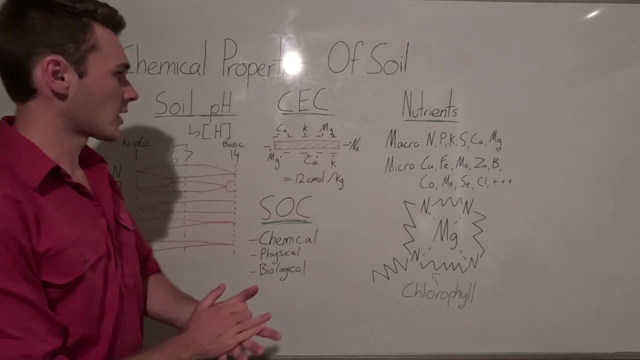 You've got to think of this as almost like a bucket for our soils to hold onto cations. Now, cations are nutrients in our soil that have a positive charge, So calcium, potassium, magnesium, sodium to some extent, And so the way our cation exchange capacity works is that we have a negatively charged particle in our soil called a colloid. 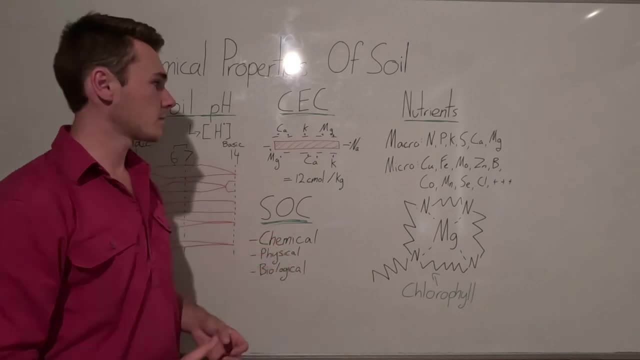 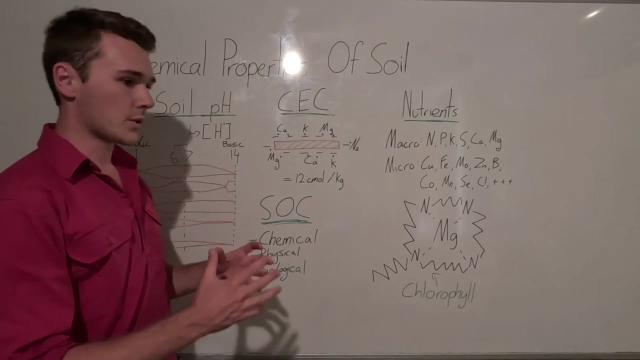 And this colloid, as I said, has a negative charge to it, And so it's going to, It's going to attract these positively charged ions, or they're called cations, And so the greater this negative energy within our soil, the greater the amount of cations that can stick to it. 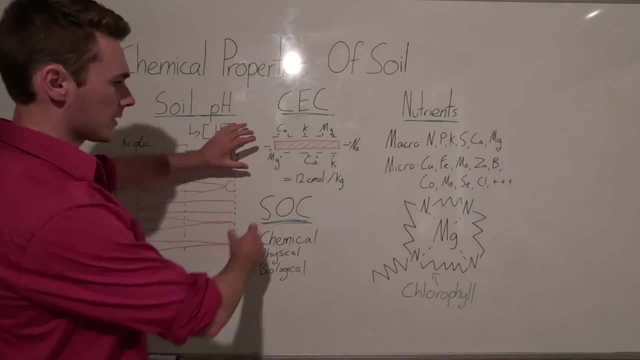 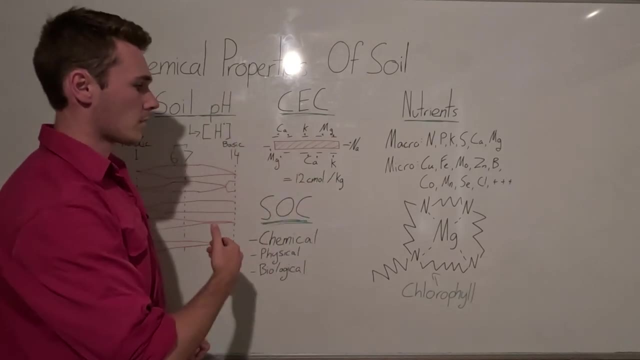 And so if you think of almost like a magnet in our soil, that's going to have our negative sites And then we can have our positive cations clinging to that, And so this is usually expressed in centimoles. Mole is just a number. 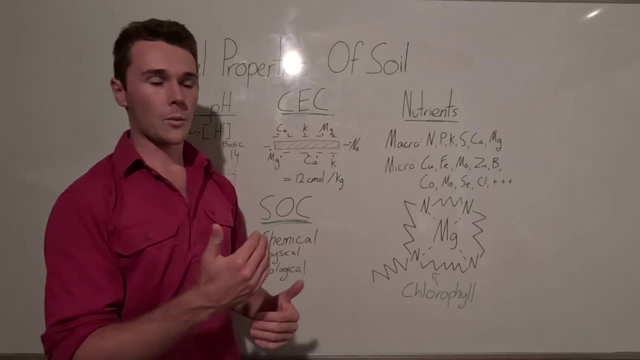 It's similar to saying, like having a positive cation, I mean a dozen eggs, one mole is. it's a pretty large number, but it's just saying that there's X or there's that many of this particular thing. 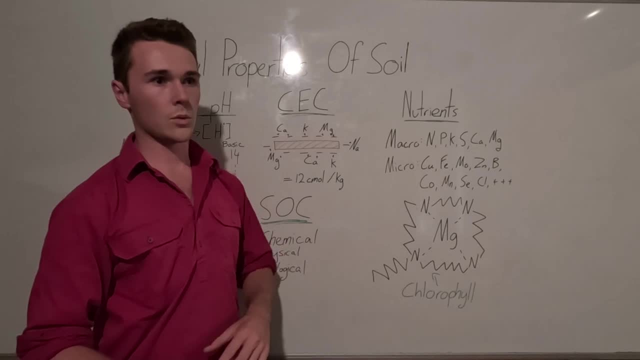 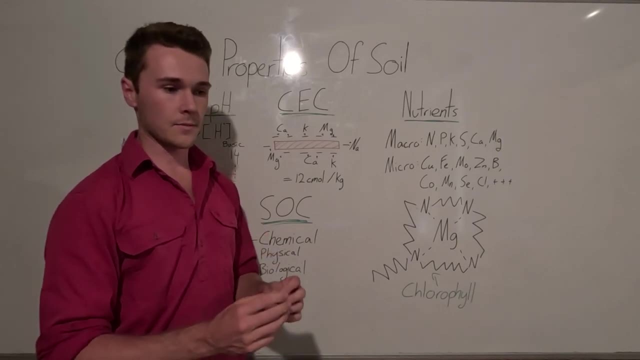 So a mole in itself is, I think it's- 6.02 times 10 to the 23. So that's a massive number And it's usually used to describe um elements and things of those chemical natures. So really small scale. 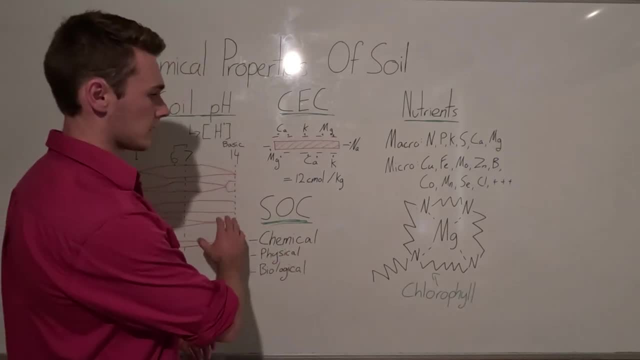 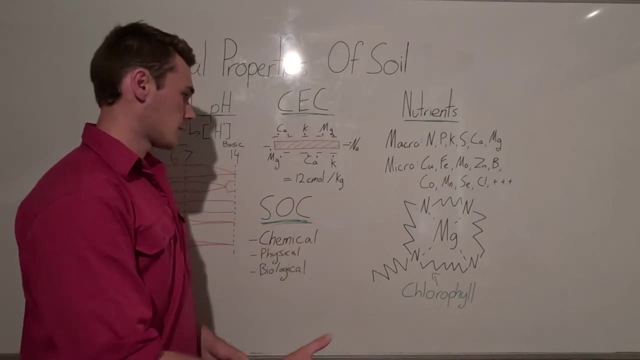 And there's a lot of them. And so instead of saying you know, there's trillions and trillions and trillions of things in our soil, we say there's a couple of mole. Anyways, it's like a dozen. 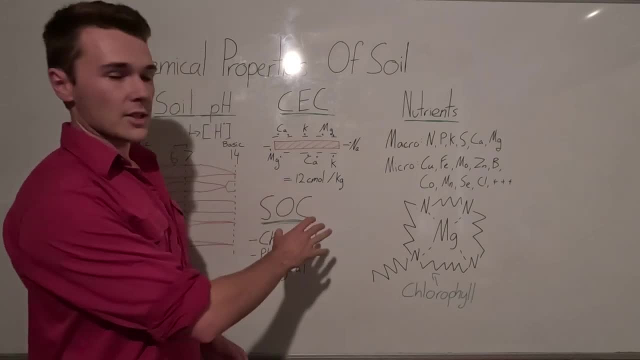 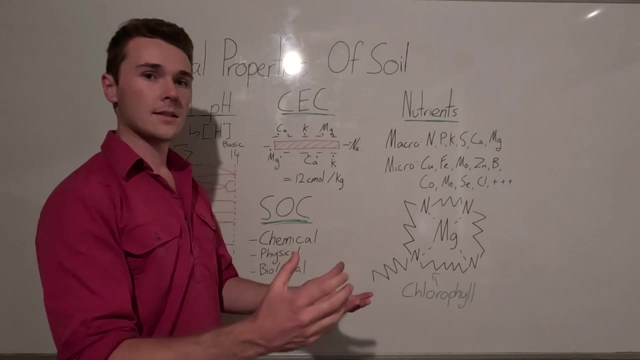 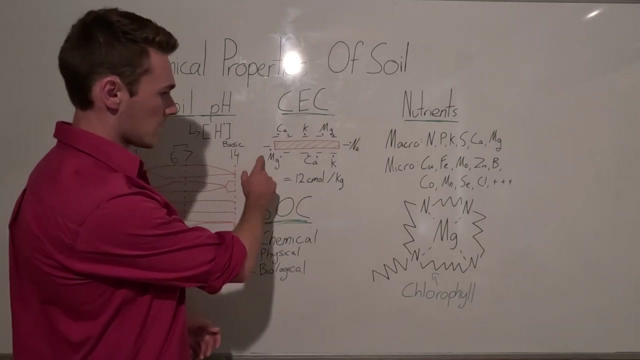 So we express our cation exchange capacity as centimoles per kilo. So per kilo of soil, how many positive things can we stick in that? And so for this one here, for example, it's 12 centimoles per kilo, which means there's basically 12 centimoles of cations that can stick to one kilo of soil. 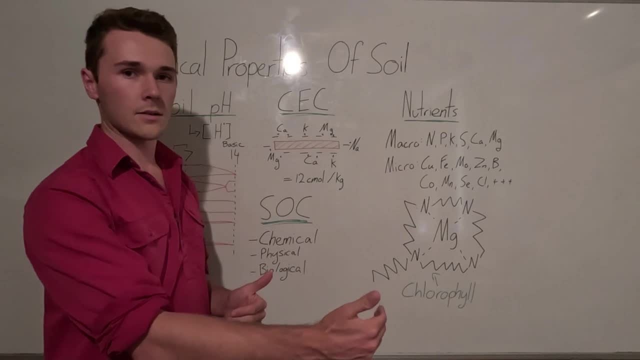 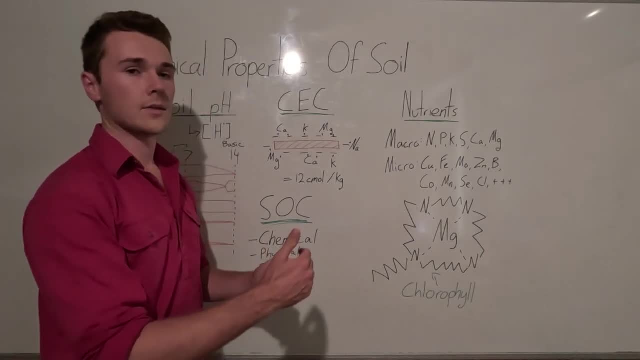 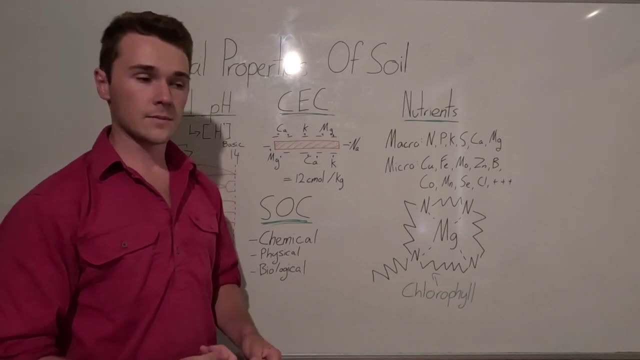 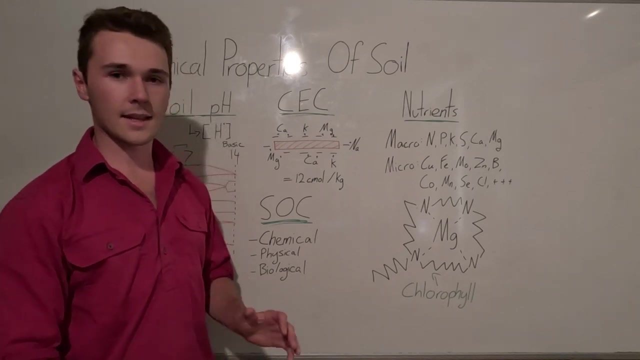 The lower your CEC, the worse and often less fertile your soils are. So the only particles that have a CEC uh are clay particles and um organic matter. Everything else doesn't So uh clay. so sand and silt doesn't have anything.